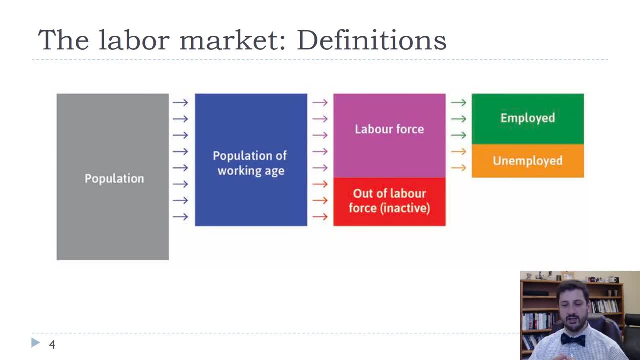 Some countries might also take out people of retirement age, although more and more people over 65 in the United States are working, Then we can divide up the population of working age into the labor force and out of the labor force. People out of the labor force would include people who are retired. 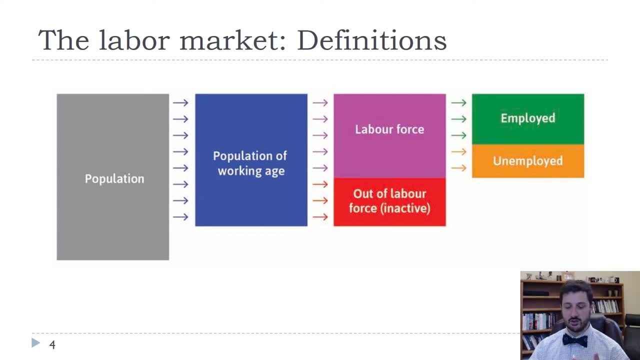 people who are parents taking care of their kids and not looking for paid work, students not looking for paid work, anybody who's not looking for work. Then we can divide up the labor force into two groups: the employed, which is our green box here, and the unemployed. 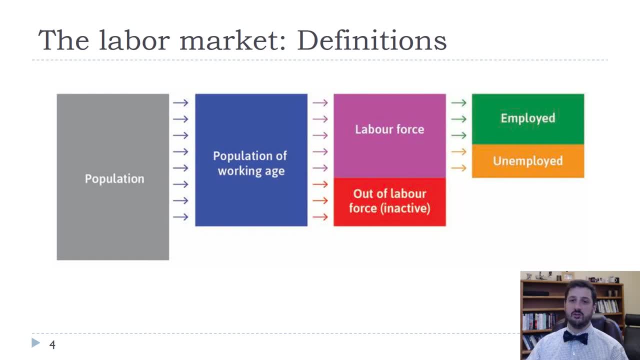 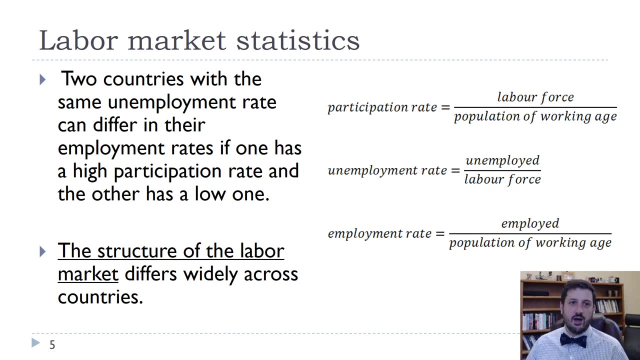 so everybody in the labor force wants to be working, but not everybody is working. We're going to look at a number of labor market statistics. We can see that there are a number of differences in how countries' labor forces are divided up. We can look at the participation rate, which is everybody who wants to work the labor force. 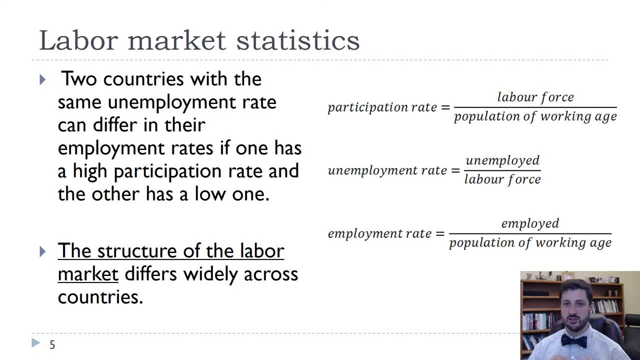 divided by everybody who could work, which is the population of working age. We can look at the employment rate, which is the unemployed divided by the labor force. Remember, the labor force is employed plus unemployed, so it's unemployed divided by employed plus unemployed. We can also: 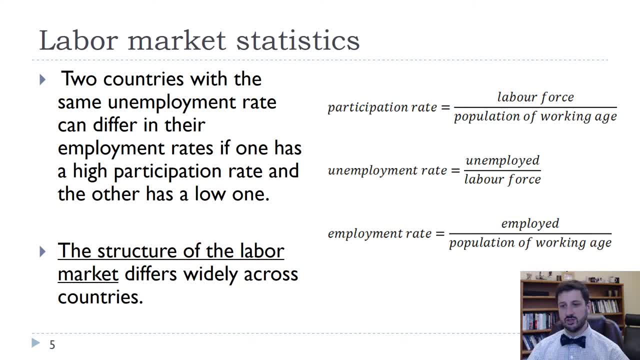 look at the employment rate- the employed divided by the population of working age. so how many people who could be working are actually working? There's a number of different outcomes depending on the country. They have some examples, for instance, comparing some of the. 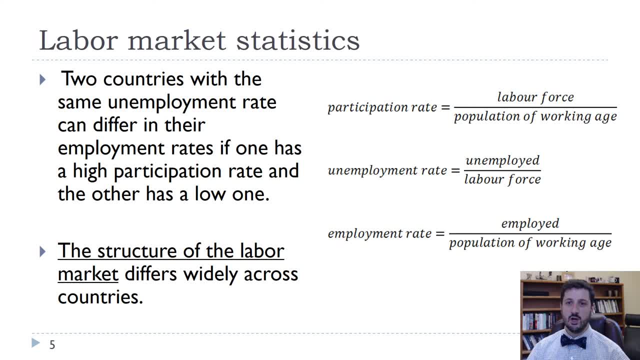 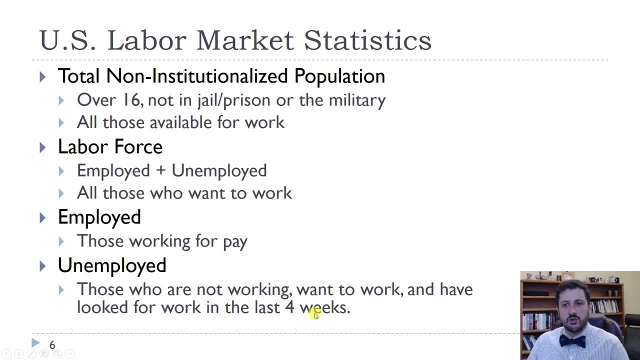 countries to some of the Southern European countries, where the Nordic countries seem to have much better institutions in terms of keeping the unemployment rate lower, keeping the employment rate higher than some of the Southern European countries. If we look at the United States, the way we frame these populations is just a little bit different. We look first at the total. 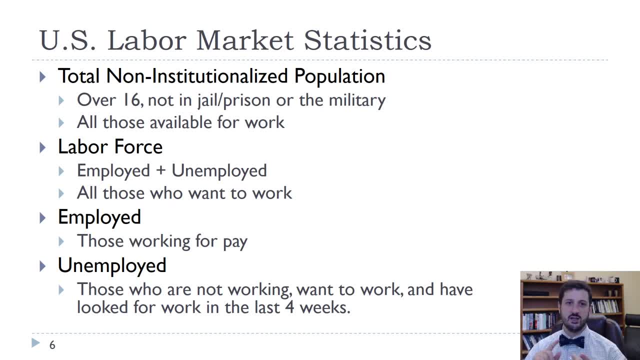 population, and so that's people who are over 16, not in jail or prison or the military, and we can think of that group as everybody who's available for work. Then the labor force is the same. It's the employed plus the unemployed, so all of those people who want to work. 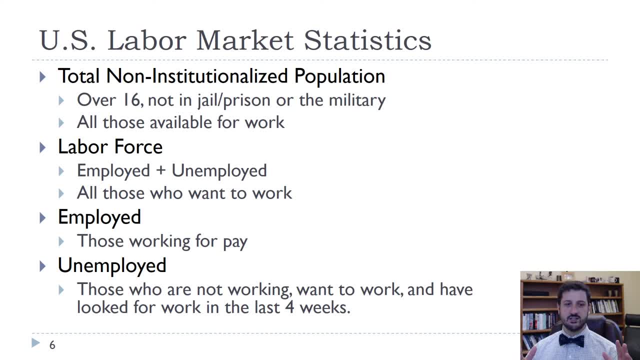 Employed are those working for pay, and the Bureau of Labor Statistics, which is the organization that measures all of these statistics, defines the unemployed as those who are not working, who want to work and have looked for work in the last four weeks. It's based on a survey. 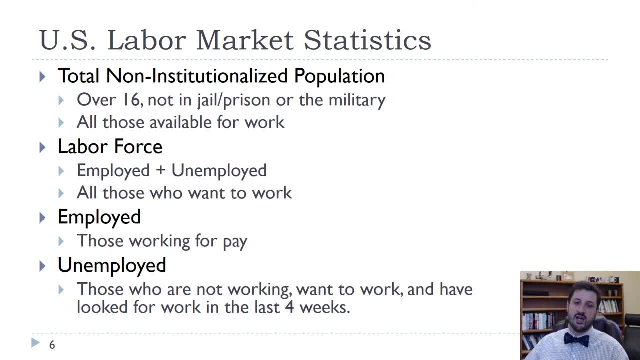 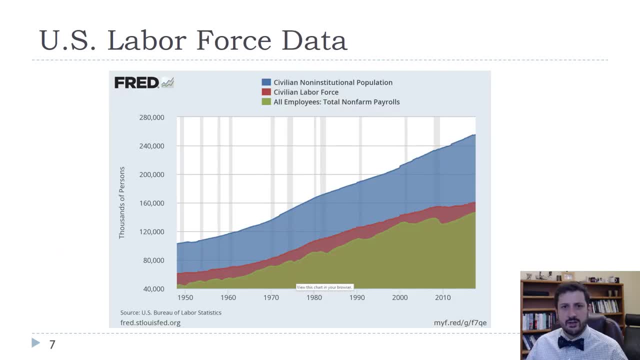 of households and if you haven't looked for work in the last four weeks, then you're not counted as unemployed. We can look at these numbers. The blue line measures the civilian, non-institutional population. You can see that currently it's around 250 million people. 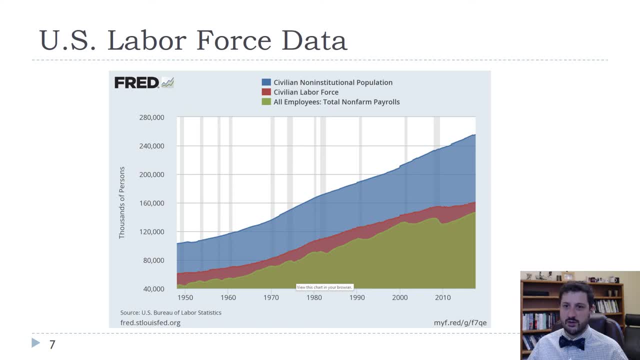 The red line is the labor force, and so that's around 160 million people. The green line is all the employed people. The difference between the red line and the green line, then, would be the unemployed people, and you can see it increased here during the Great Recession. 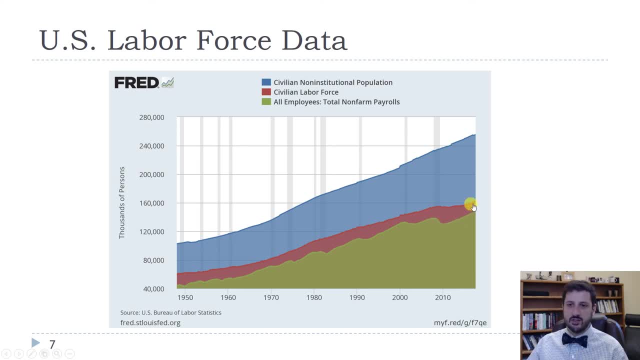 in 2008-2009, then started recovering and the unemployed is still relatively low. but you can also see that the group that's not in the labor force, which is the difference between the blue line and the red line, has been increasing, and there's been a couple of reasons for that One. 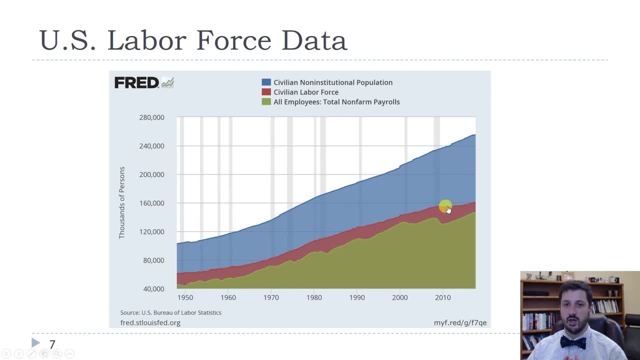 is that we're getting older, and so we have more people in that age- 65 and above range, as the baby boomers retire, and also because the labor market still hasn't fully recovered, and so the labor force participation rate, which is the red line divided by the blue line, has been falling since. 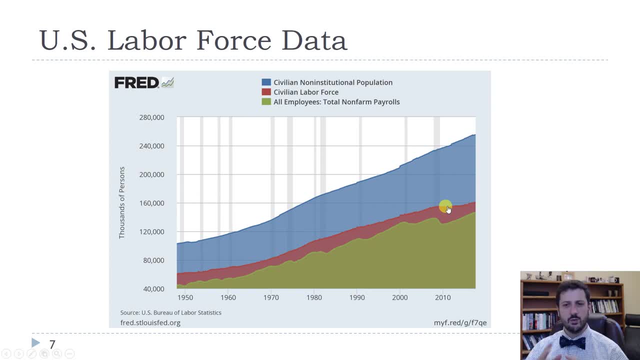 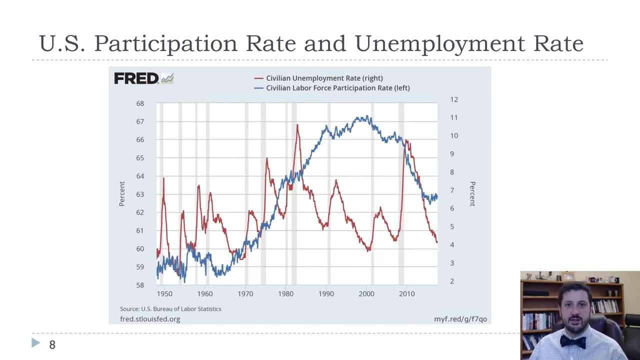 about the year 2000,. and we're not completely sure why that is. If we look at the civilian labor force participation rate, which is the blue line but measured on the left axis, and the unemployment rate, we can see that there is some relationship between them. The 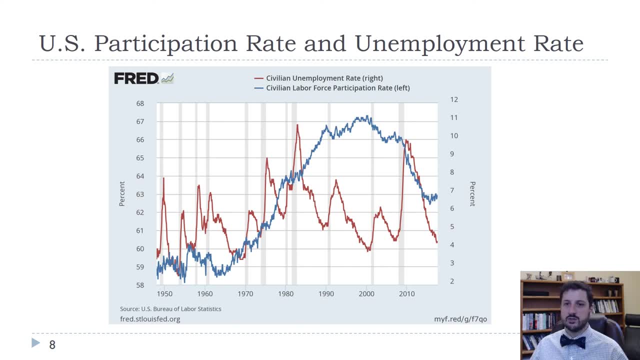 participation rate tends to fall. when the unemployment rate goes up, People stop looking for work. They might decide, all right, I'll just be a stay-at-home parent. They might just give up looking for work. They might decide to go back to school. but we can also see that, since